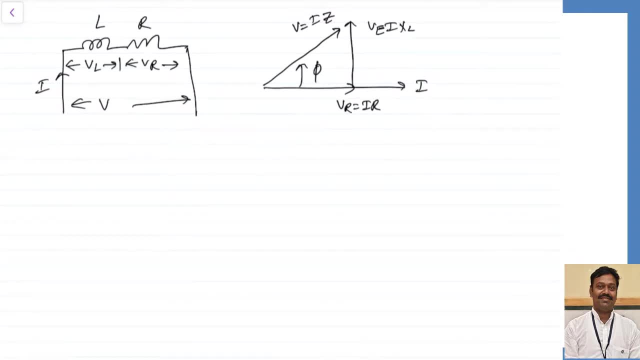 the current respect to current by some angle, phi or otherwise, we can tell this voltage v is the sum of the voltage because of the resistive circuits plus voltage because of the inductive. so otherwise we can tell that this will become equal to i into r whole square. this is i into. 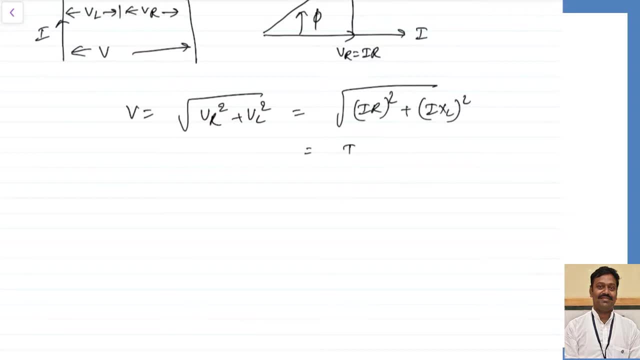 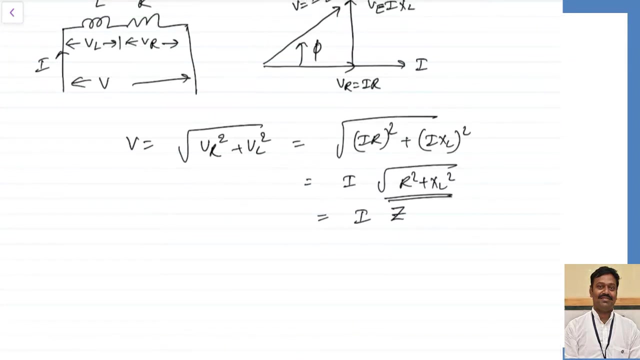 xl whole square, or this i can write as i into square root of r square plus xl square. so this i can write as i multiplied by z, where the square root of r square plus xl square is called as immutable impedance of the circuit. so to calculate the angle phi, this phi i can calculate as tan inverse of. 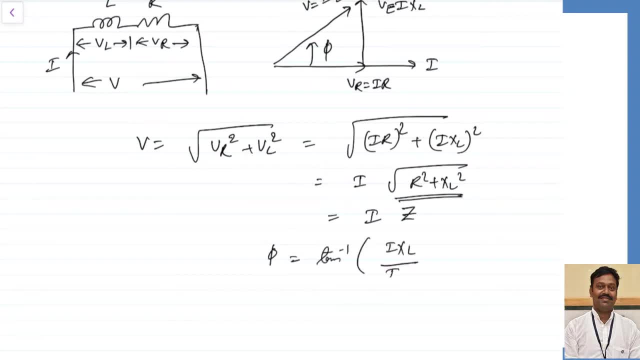 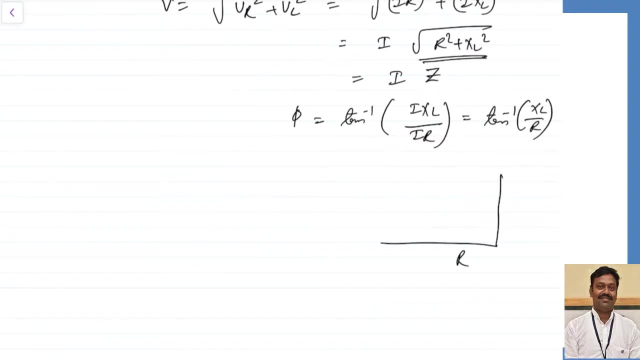 y component by x component. this is i into xl divided by i into r. i can get from this circuit so this will be equal to tan inverse of xl divided by r or this. using this i can develop one impedance diagram. so i can write this in this form. this r is the x-axis, x component, and 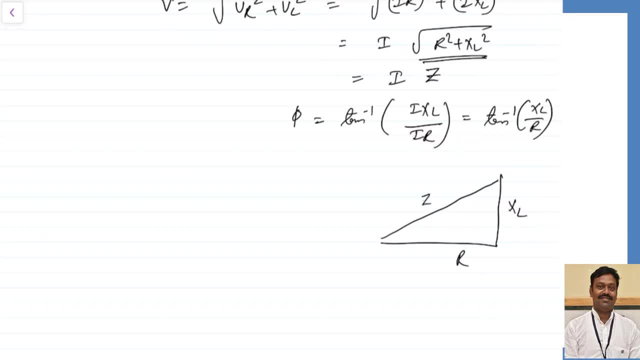 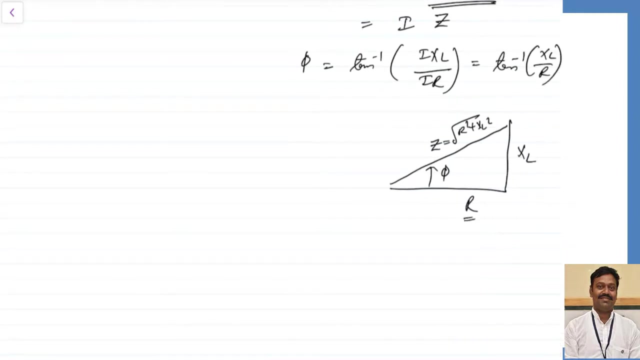 the y component is xl, then automatically this resultant will be equal to the impedance of this joint. so i will anything else that we have. that means we are known dip saw as y minus in cube. so we can write: this is a linear movement of x-axis f, which is equal to log x is what we will write, the inverse of x. 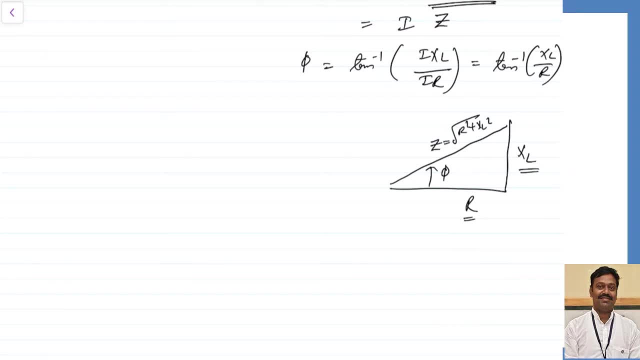 which is y plus x. so people here have to keep in mind that we need to have this linear movement right and we can write r plus j- xl. that means i can write the z is equal to r plus j into xl. or i can write the z is: 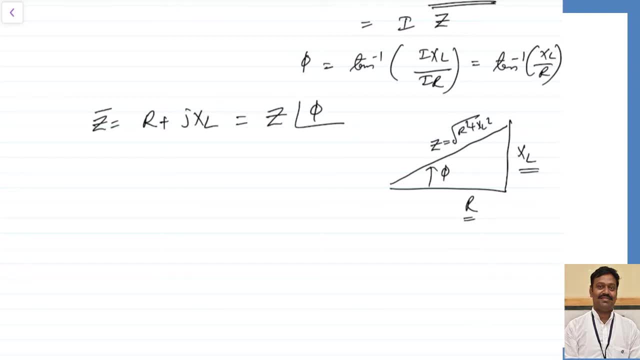 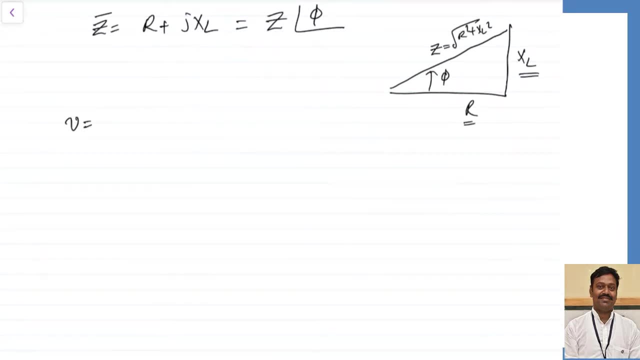 nothing but the z at an angle of some angle, phi, where phi is tan inverse of xl divided by r. so let us try to calculate the power. we know the instantaneous value of the voltage. if you are taking voltage as my reference, i can write as: v maximum sine omega t. so if voltage is taken as: 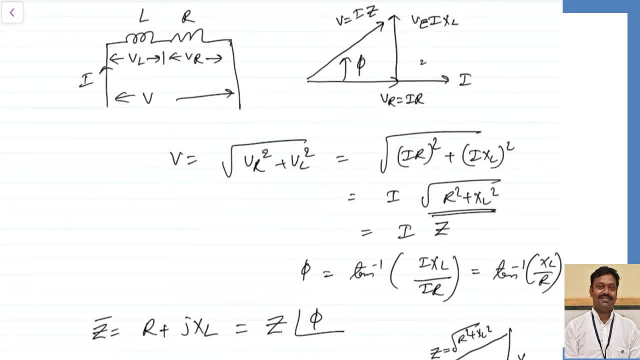 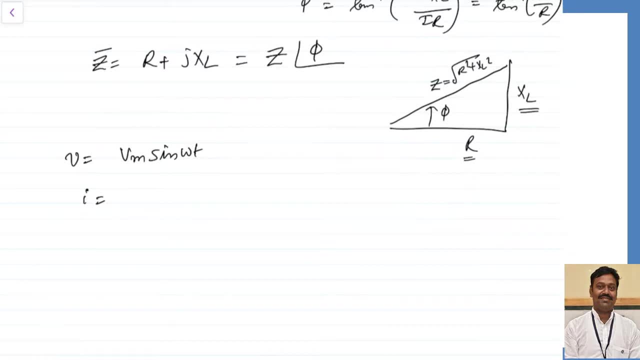 reference because we have taken the current as reference. we got my voltage leading the current by some angle phi. if you are taking the voltage as reference, we can tell that current is lagging the voltage by some angle phi. so i can write it as i: maximum sine of omega t minus phi. so if you 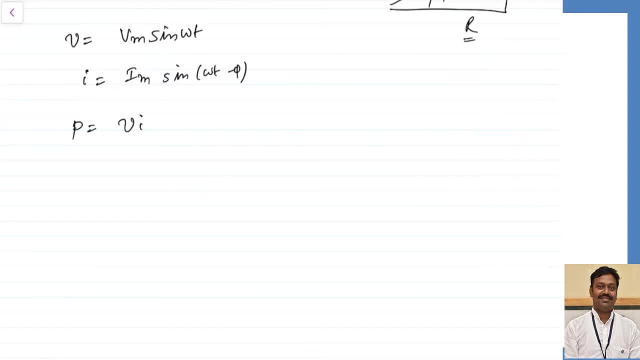 want to calculate the instantaneous power. instantaneous power will be instantaneous voltage into instantaneous current. this will become v maximum sine omega t into i maximum sine omega t minus phi. so this i can write as v maximum, i maximum i am dividing by 2 and multiplying with 2, so this becomes sine. 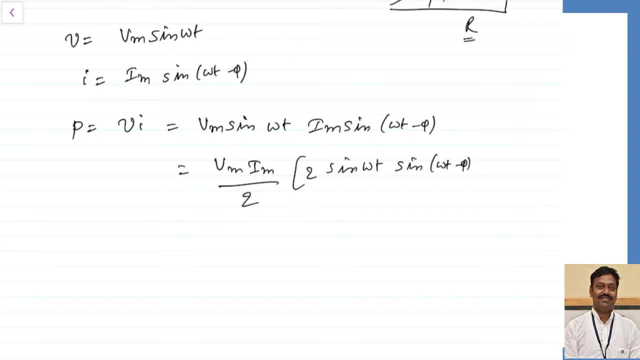 omega t sine of omega t minus phi. this is what we got. so 2 sine a sine b. i can write of the form cos a plus b minus, cos a minus b- sorry, this is minus. sign will come right like cos a minus b minus. cos a plus b will give my value of 2 sine a sine b. so this i can write as v maximum i. 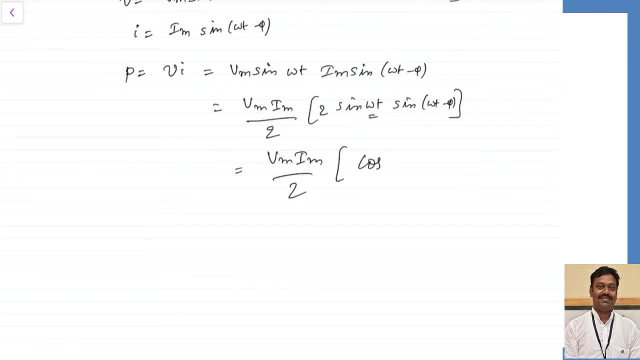 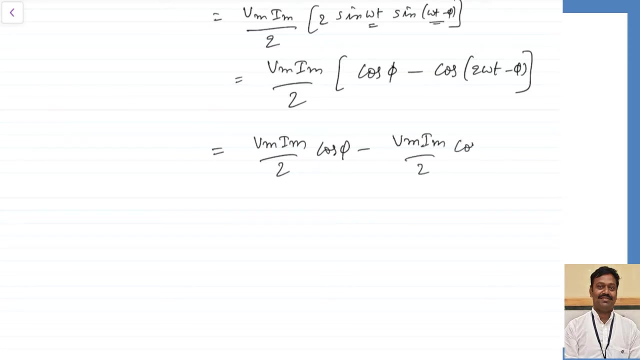 maximum by 2 into cos of omega t minus omega t minus phi. this will become cos phi minus cos of a plus b. this becomes two times of omega t minus phi. so i have just converted this, so this i can write as v maximum i maximum by 2 into cos phi minus v maximum i maximum by 2 into cos of two times of omega t. 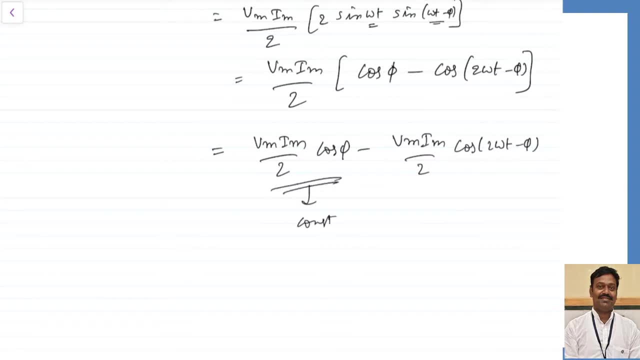 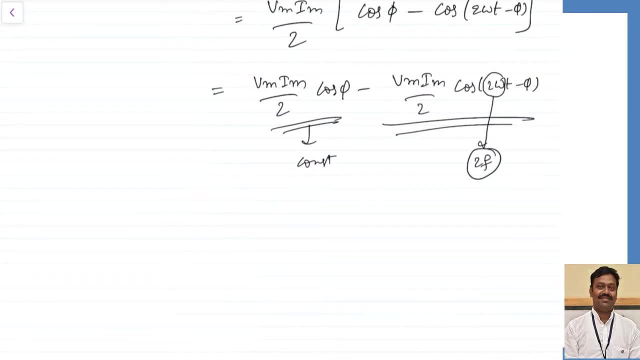 minus phi. you can see, this term is a constant term and the second term is a term which is oscillating at two times the frequency. so, which is oscillating at two times the frequency, that means in one half cycle it completes one full cycle. so now, if you want to calculate the average, 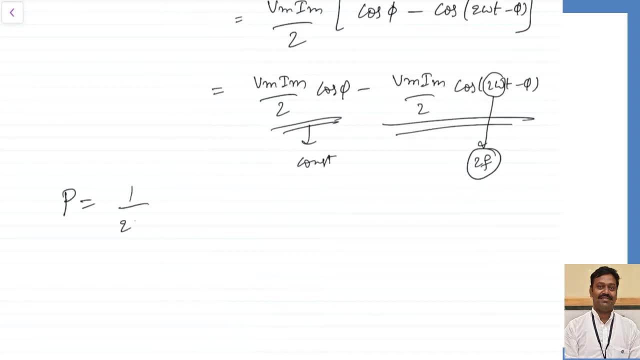 power. average power will be equal to average for the full cycle. so i have to take from integration from 0 to 2 pi into whatever is p. this i have to write d omega t, so this i can write as if you just solve this, and then you can write this as v maximum by 2 into cos phi minus omega t minus phi, so this: 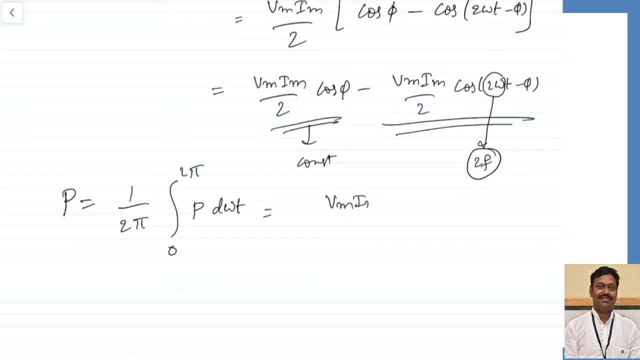 integrating from 0 to 2 pi, you will see that only first term will remain. second term will become 0 because it is oscillating at double the frequency. so the average will be equal to 0. so this becomes v maximum- i maximum by 2. into cos phi, or this i can write as: v maximum by root: 2 i maximum by root. 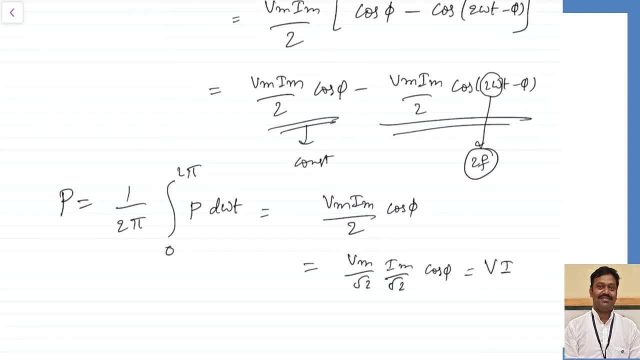 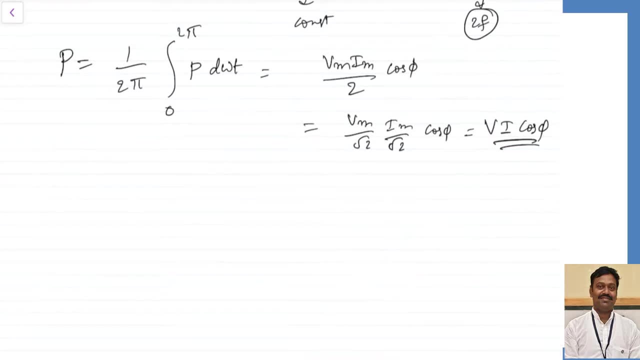 2 into cos phi and from this we got this is v, rms, irms into cos phi. this is what we got. this v into i into cos phi is giving my active power. so let us try to write the active power. so p i can write as v into i into cos phi. so from the impedance triangle i can represent the value of cos phi. 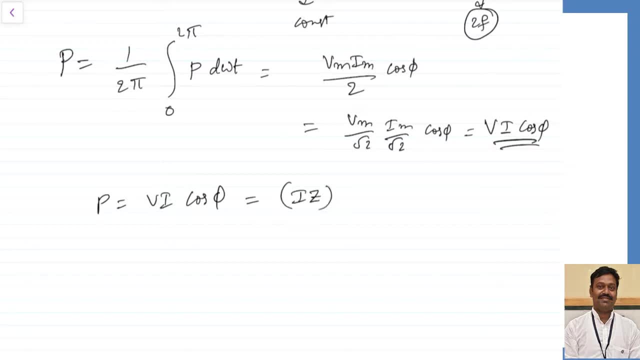 so i can write: v is nothing but i into z multiplied by current. i multiplied by cos phi is nothing but r by z, as per impedance triangle. this is my r, this is my x and this is z, this is my angle phi from the impedance triangle, cos phi is adjacent by hypotenuse, so r by z. 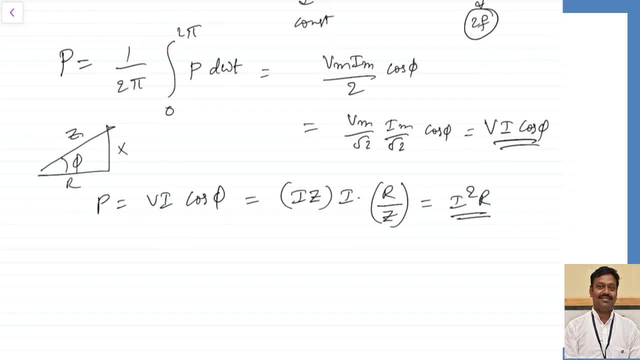 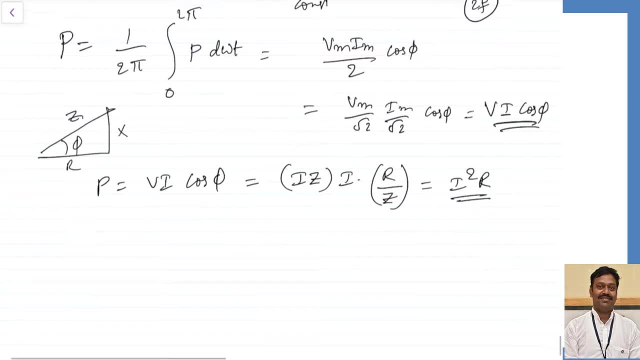 So if you calculate this you will get I square into R Or. from this we have proved that whatever the active power is lost, that power is lost only because of the resistor and the inductor does not consume any power. One quarter cycle it takes the power. Another quarter cycle it returns back the 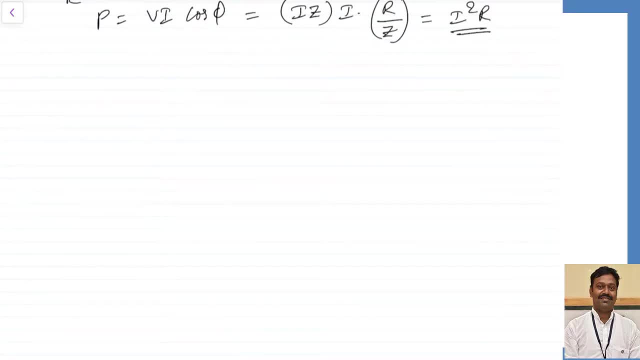 power. So this is what we have studied. So from this we have summarized previously that if this is my voltage and the current is lagging by some angle, I some, I is lagging by some angle, phi. So this I can write as I cos: phi is the x component. Similarly, the y component will be equal to I sin. 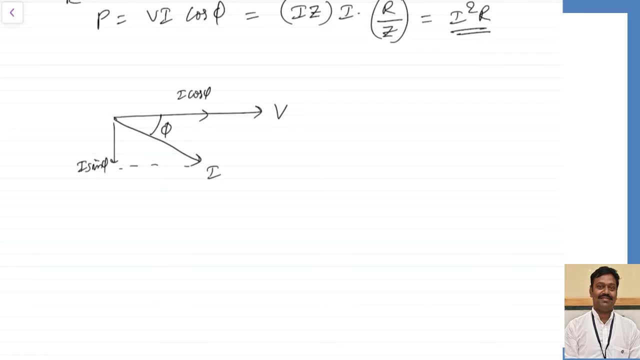 phi. So I am just multiplying both sides with the voltage V, So this becomes V into I into cos phi. This is V into I. This is V into I into sin phi. Or this I can represent in this form: V into I into. 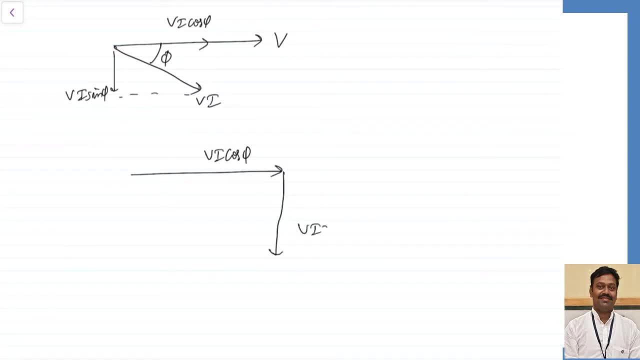 cos phi. Adding to this V into I, into sin phi, we got the value of V into I. This is what I got, So this angle is phi. So we got this. as this is my true power, So this is my reactive power and this is my apparent power. This is what we have seen from the true 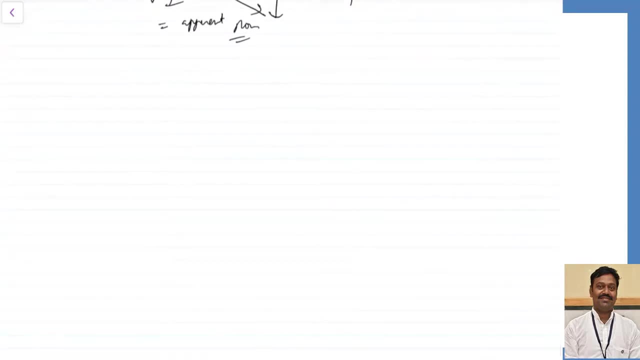 reactive and apparent power. So now I want to use the phasor algebra to calculate my value of active reactive and the apparent power. to calculate active reactive on the apparent power. so let us assume the value of the voltage v is coming like this: v is making an angle of- let us assume angle of theta 1. let us assume current. 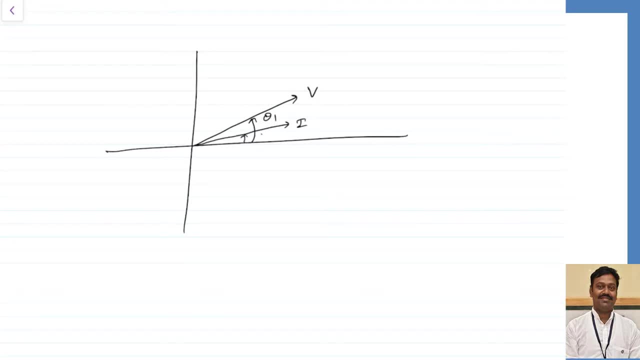 is lagging this voltage and this i current is making an angle of theta 2.. that means v is leading by some angle. so vf i am taking this- v is having an angle of theta 1 and the current is having an angle of theta 2.. so, as per the power calculation, we know that i want my power, p should. 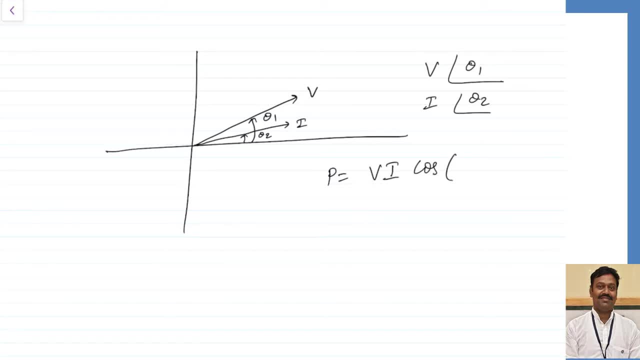 be equal to v into i, into cos of the phase difference between voltage and current. so this will become equal to cos of theta 1 minus theta 2.. this is what i want. similarly, the reactive power should be equal to v into i, into sine of theta 1 minus theta 2 and the second one. 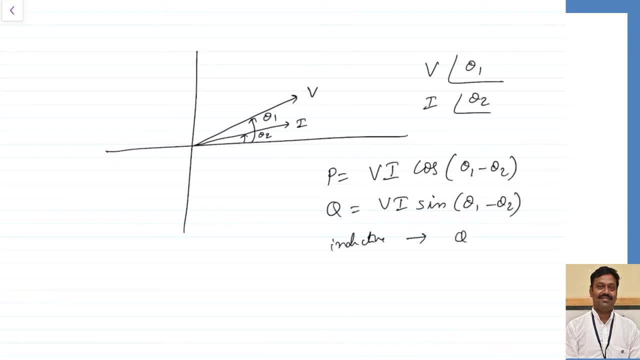 for inductive reactance. if the load is inductive, then q should be positive, and if it is capacitive, the q should be negative, because we know all our practical loads are inductive loads. so that's why, for inductive loads, it will be convenient to take the q as positive. 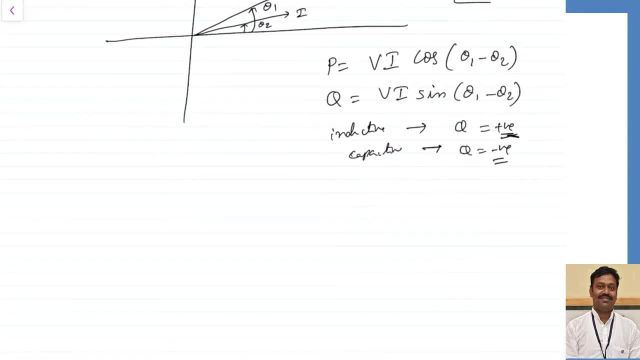 because it will be easy to do otherwise every time that minus configuration will be there. so let us try to calculate. so to calculate apparent power: s i can simply multiply v into i, let us see what will happen if i multiply v and i. so this becomes v at an angle of theta 1. 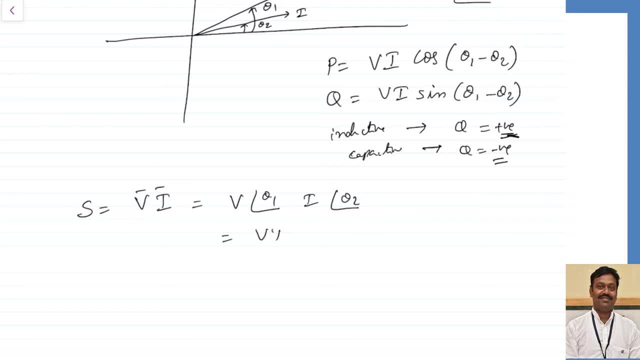 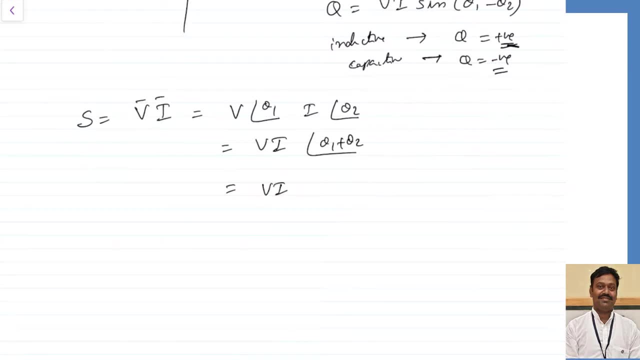 and i is having an angle of theta 2, so this will come v into i at an angle of theta 1 plus theta 2. you can see it is adding the angles, not subtracting it, because you can just convert this to rectangular form: v into i, into cos of theta 1 plus theta 2. 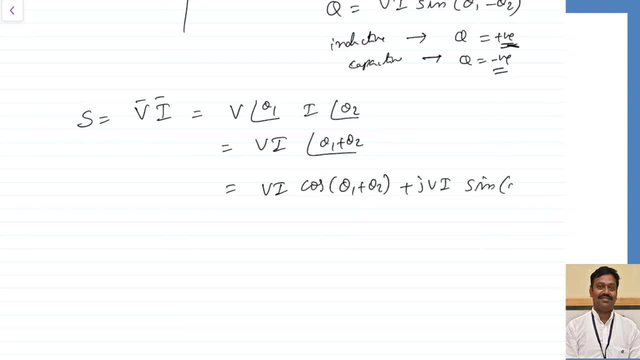 plus j times of v into i, into sine of theta 1 plus theta 2. you can see this is also not correct. this is also not correct. but actually i want the difference of the angles. so that means if you want to get the difference i have to take conjugate of one of the vector. conjugate means only angle. 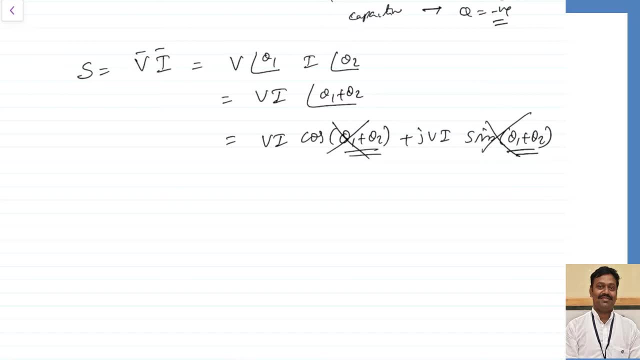 will change. magnitude will remain same. this we have already discussed before. so let us see what will happen. if i am taking the conjugate of the voltage and not the current, so this will become v at an angle of angle, become absolute v at an angle of minus theta 1 and i at an angle of theta. 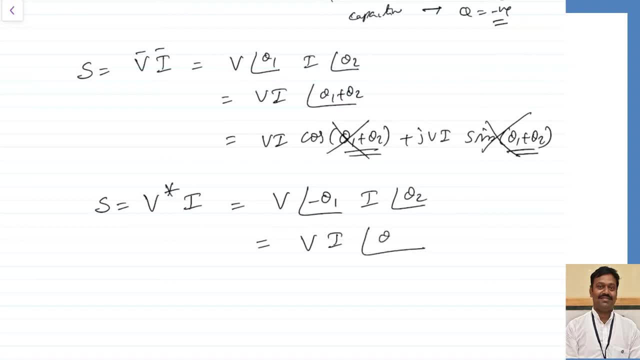 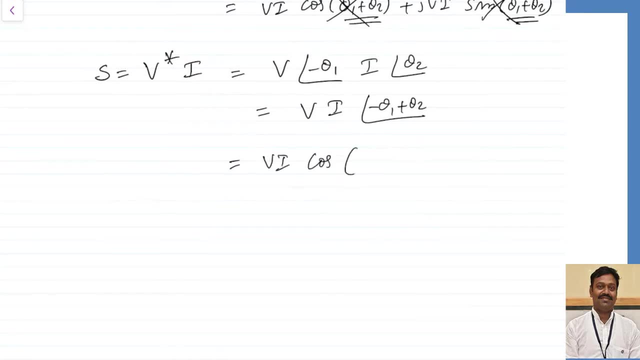 2, so this will become v into i at an angle of minus theta 1 plus theta 2, or this i can write in rectangular form: v into i into cos of minus theta 1 plus theta 2, so this will become v into i at an angle of minus theta 1 plus theta 2. 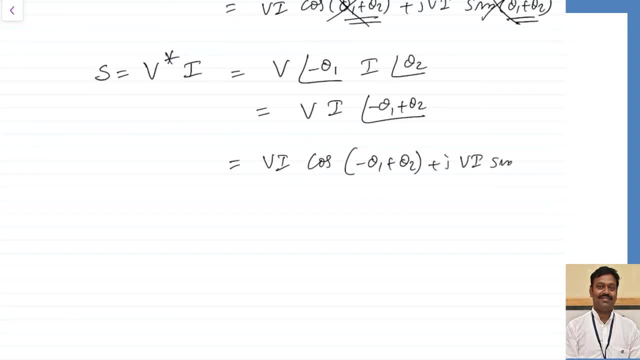 plus j's into v, into i, into sine of minus theta 1 plus theta 2. this is what i get. so this i can write as v into i into cos of minus theta will be equal to cos theta, so i can just reverse this. this will.